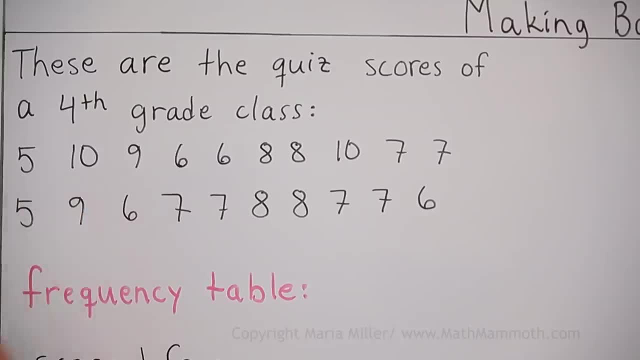 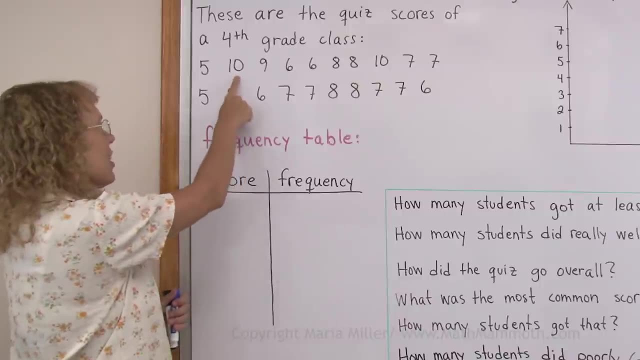 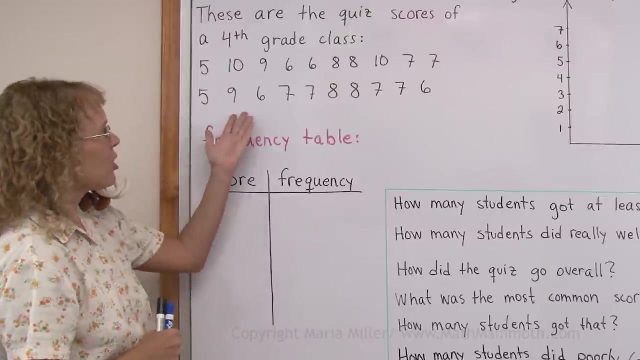 of it as a math quiz And these are the scores. So, for example, 5 means that one student got 5 in the quiz, Another student got 10.. A third student got 9, and so on, And so we want to make a bar graph out of this information. here We have to start out by making something called. 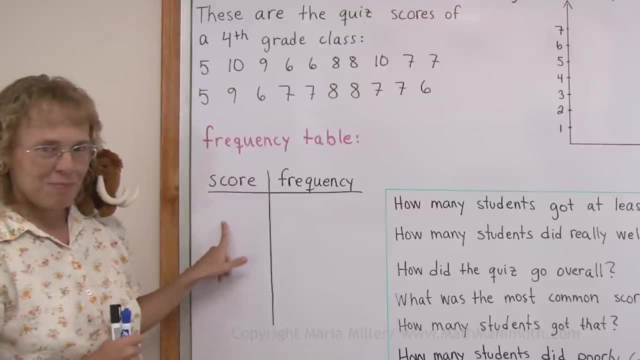 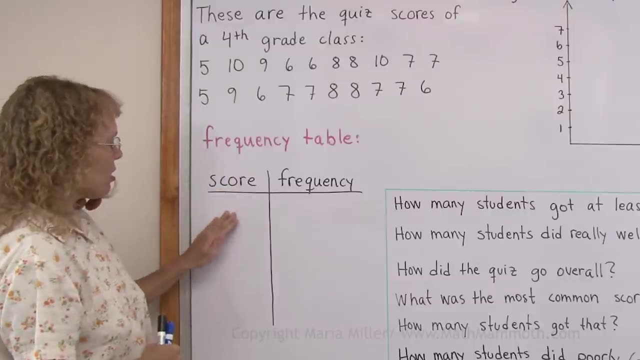 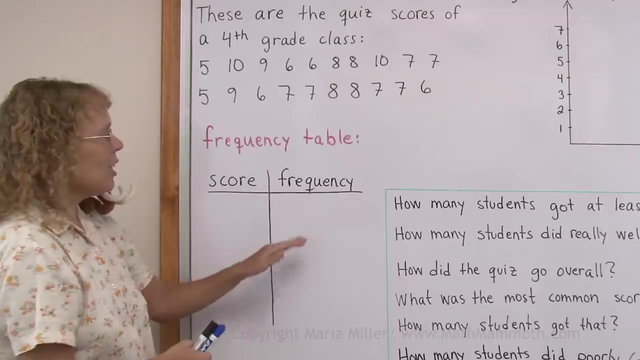 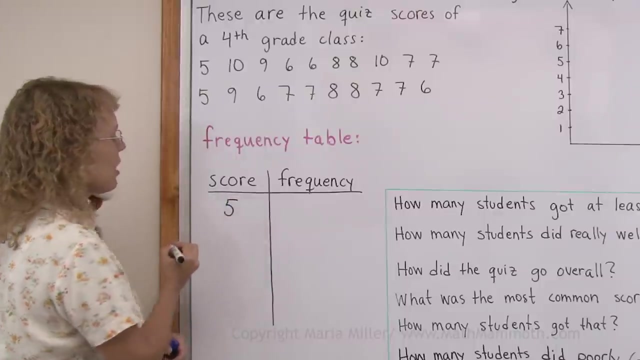 a frequency table. I'm going to make it here. I'm going to fill it in here. Frequency means how often Okay Scores are the possible scores in the quiz, Such as, you know, 5 points, 6 points and so on, And how often or how many students got that, So 5.. Some students got 5 points. 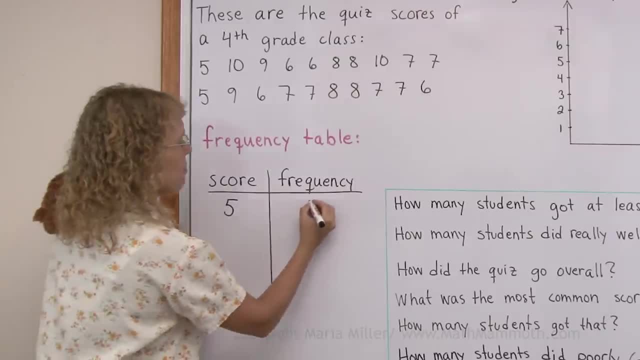 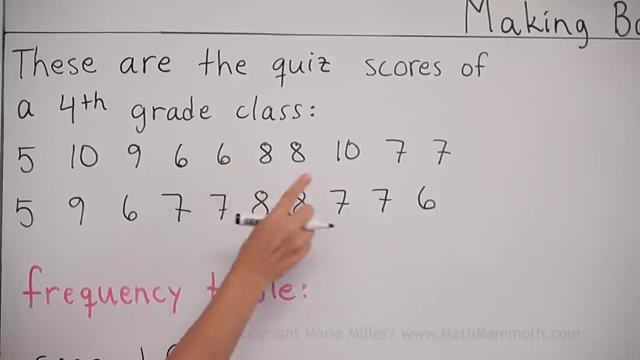 But how many 2 students, That's how often, or how many The frequency, And then 6.. We need to count here. There's 1, 2, 3, 4, 5, 6, 7,, 8,, 9, 10,, 11, 12,, 13,, 14,, 15,, 16,, 17, 18,. 20,, 21,, 22,, 23,, 24,, 25,, 26,, 27,, 28,, 29,, 30,, 31,, 32,, 33,, 34,, 35,, 36,, 37,, 38,, 39,, 40,, 41,, 42,. 43,, 44,, 45,, 45,, 46,, 47,, 49,, 42,, 43,, 45,, 48,, 49,, 49,, 50. And so we have 5 points in the quiz. So 4 students got the score of 6 points And then. 7 points. we have 2,, 3,, 4,, 6 students And then 8,, 9 and 10.. 8,, 1,, 2,, 3,, 4,, 9,, 1,, 2.. 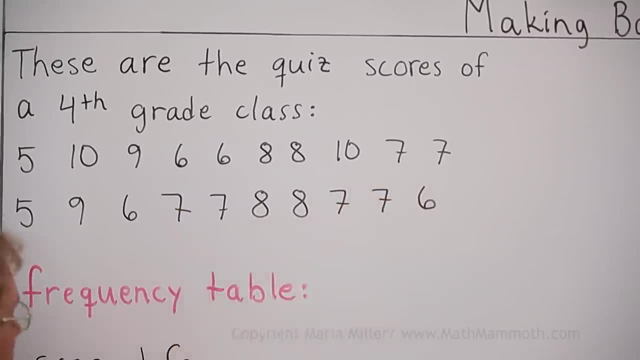 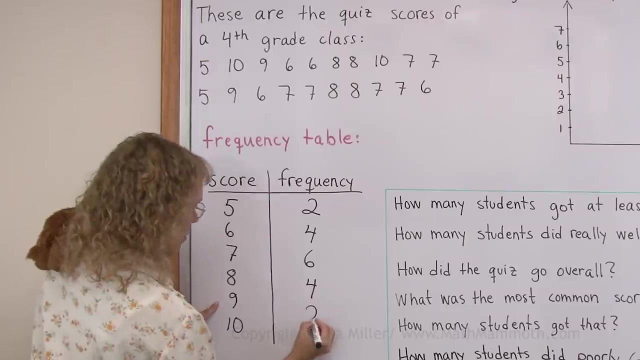 And 10, 2.. Did I get that right? Now we are ready to draw the quiz. 4 students got the score of 6 points. 4 students got the score of 6 points. six students and then eight, nine and ten. Eight. one, two, three, four, nine. one, two. 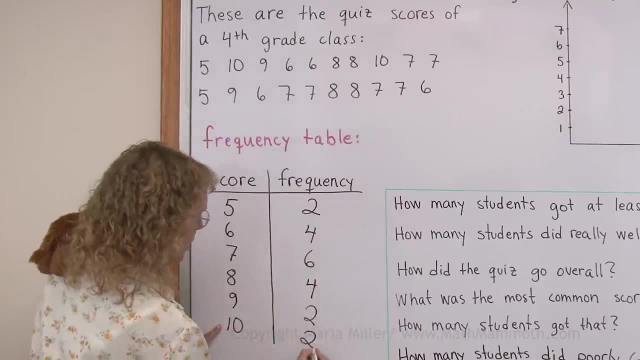 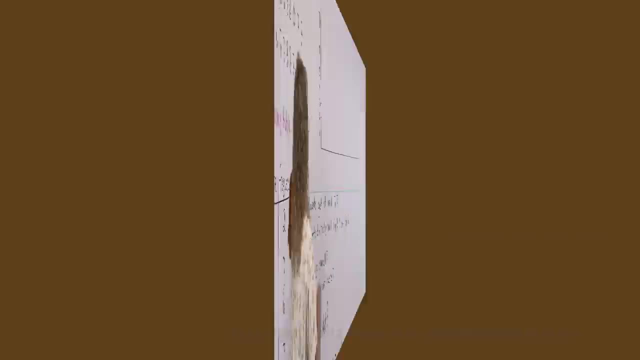 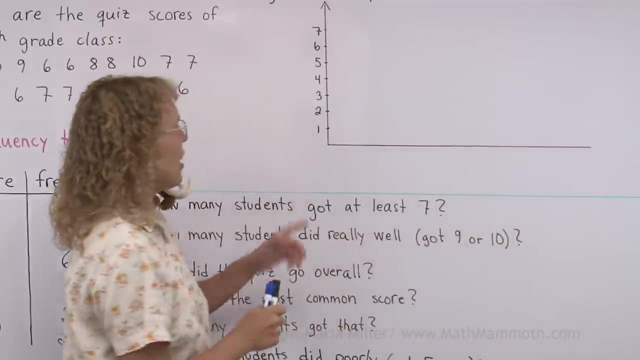 and ten two. Did I get that right? Now we are ready to draw the bar graph over there And it has a line or an axis going up this way and another axis going this way. Now these numbers here are for the frequency or for how many students. So I could write here how. 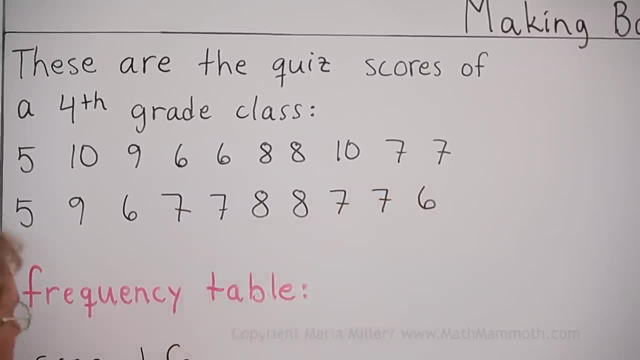 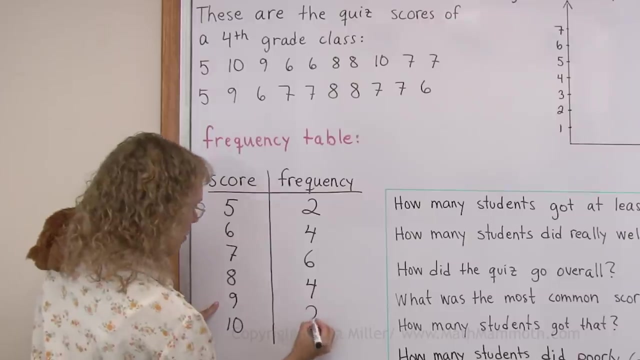 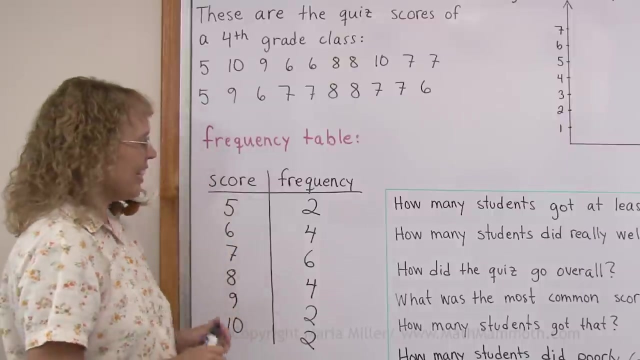 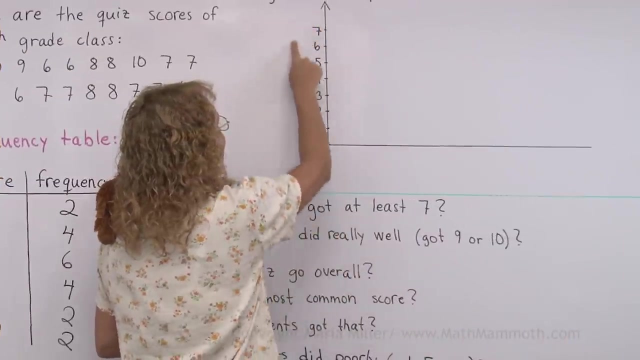 points. we have two, three, four, six students and then eight, nine and ten, eight. one, two, three, four, nine, one, two and ten, two. did I get that right? now? we are ready to draw the bar graph over there and it has a line or an axis going up this way and another axis going this way. now, these numbers here are for the. 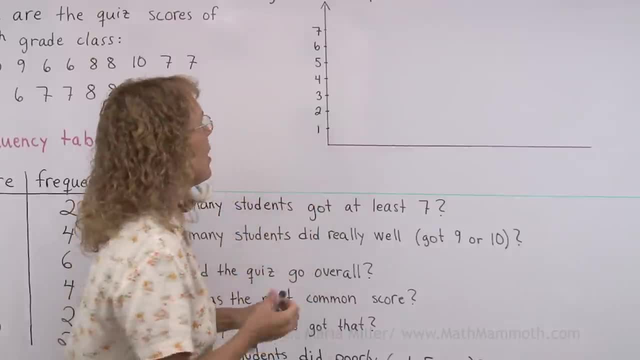 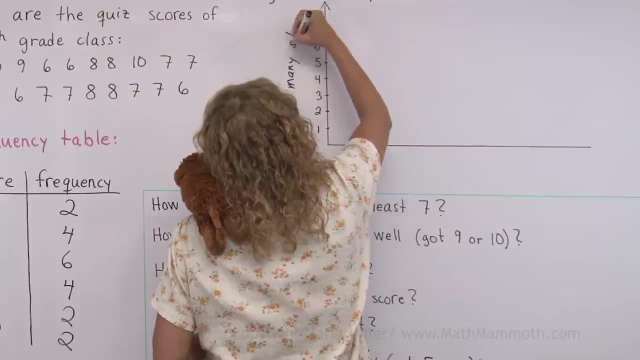 frequency or for how many students. so I could write here how many students, or I could write here frequency: I'm gonna write this time how many students. and over here go the possible quiz scores, such as we've got a number here and a number here and a number here and a number here. 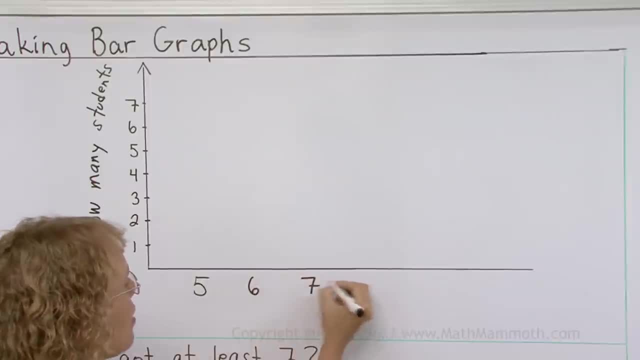 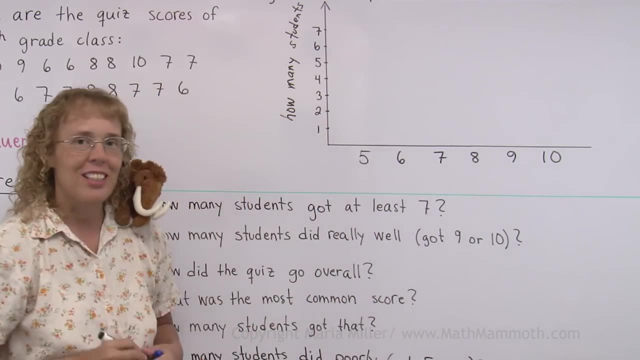 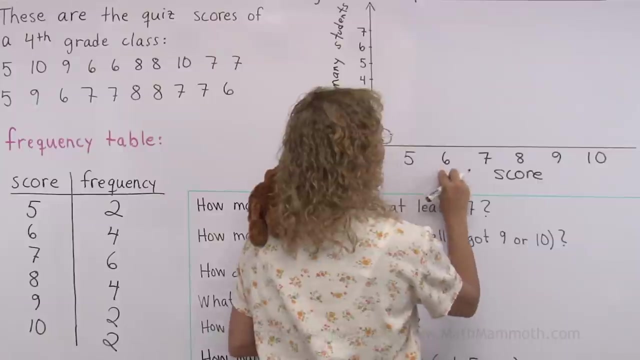 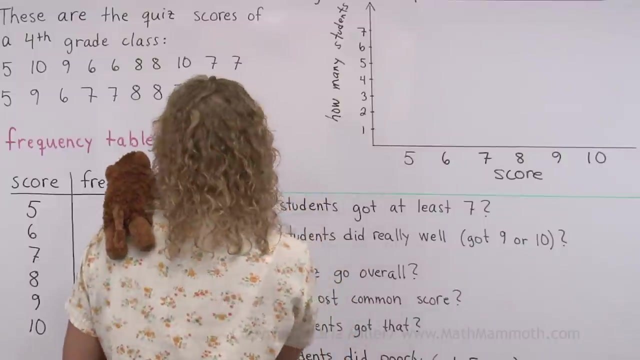 we're starting with five, six, seven, eight, nine and ten. for each of these I will then draw a bar or a rectangle. and let me add one more thing, which is score. these are the possible quiz scores, and so how many students got five points? we read in our table. there was two students, so now we draw the rectangle here and 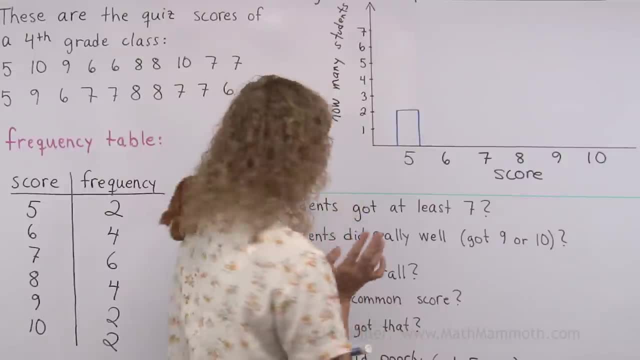 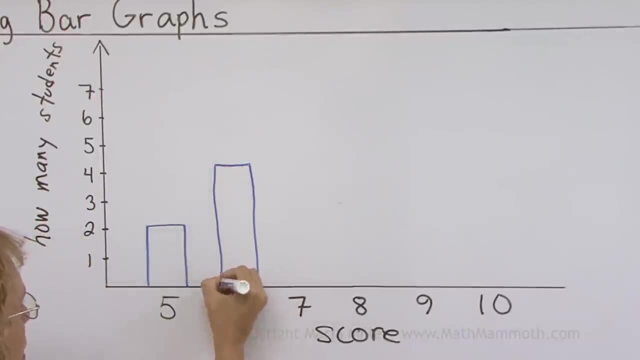 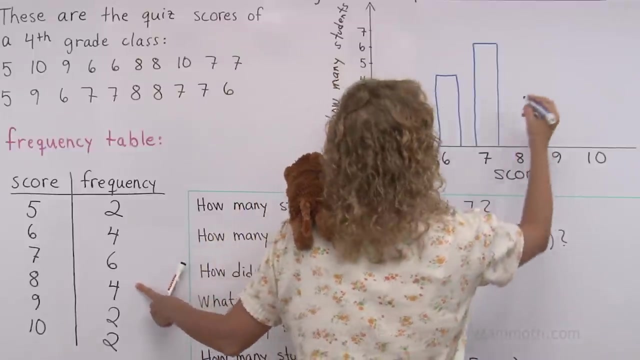 then how many students got six again looking over there for students, so now this time we need to draw it for high- and then seven, six students- okay, that's was quite many. and then eight points- how many students got that here at four again? and then, lastly, two students got four points and then seven, six students. 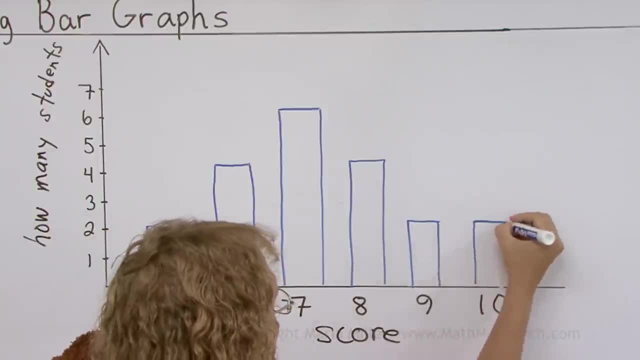 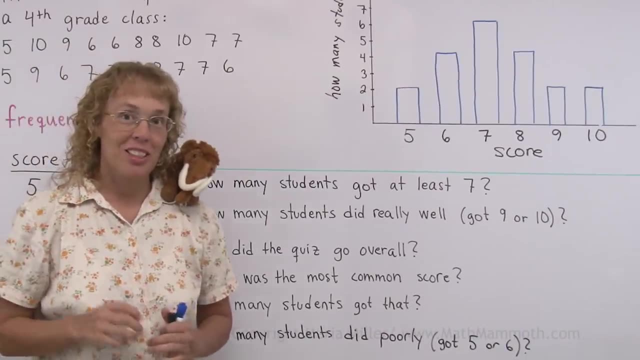 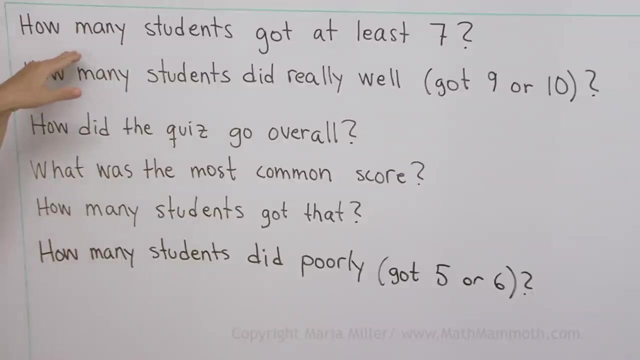 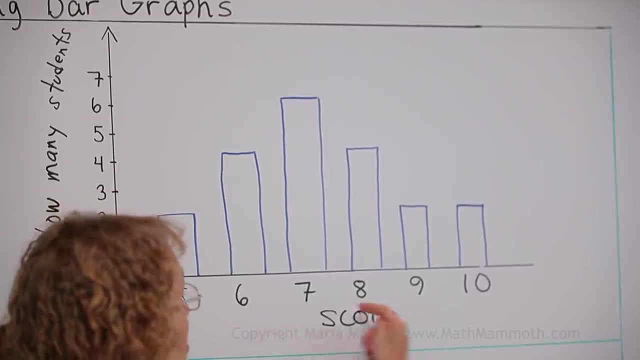 and then they all got nine and two students got ten. okay, and if you want to, you can color these in with pretty colors. now, lastly, we're gonna solve these questions here. they relate to the graph. how many students got at least seven? at least seven points? okay, they got seven points or more. that's what it. 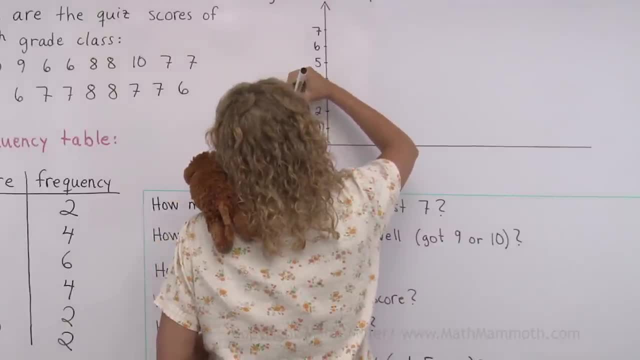 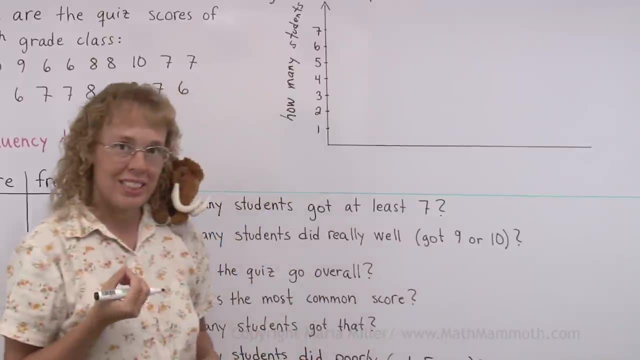 many students or I could write here frequency. I'm going to write this time how many students? And over here go the possible quiz scores, such as we were starting with: five, six, seven, eight, nine, ten, eleven, twelve, thirteen, fourteen, fifteen, sixteen, nineteen, twenty. 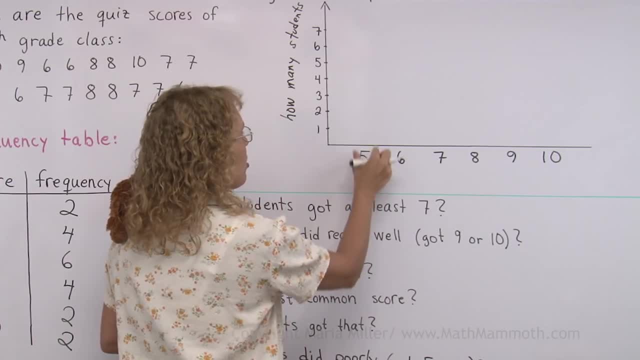 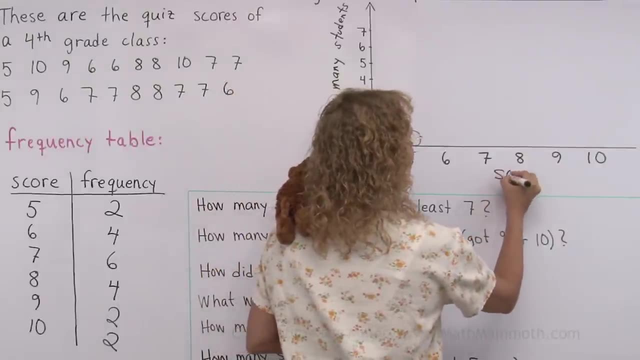 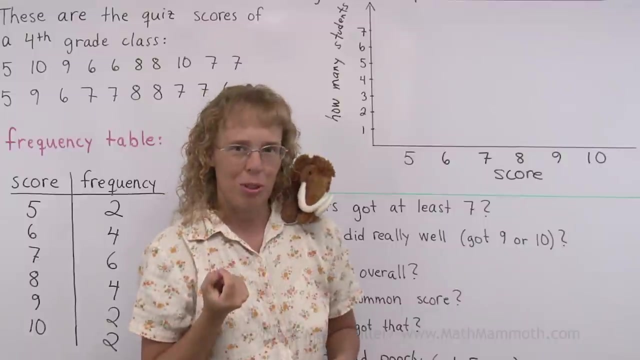 twenty-eight, ninety-nine and ten. For each of these I will then draw a bar or a rectangle. And let me add one more thing, which is score. These are the possible quiz scores. And so how many students got five points? We read in our table, those two students. So now we 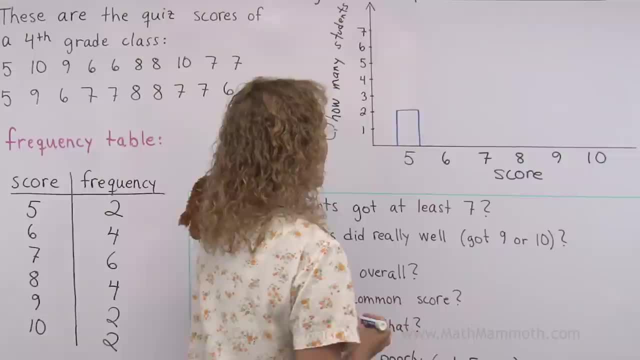 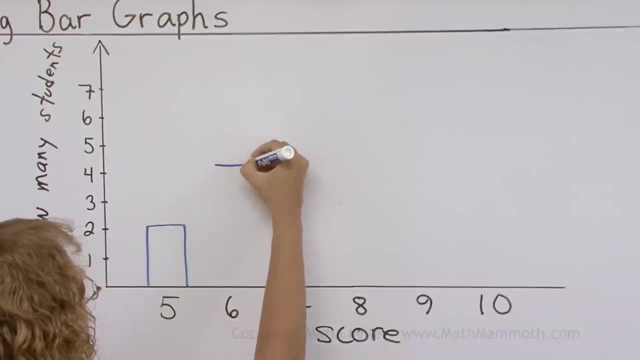 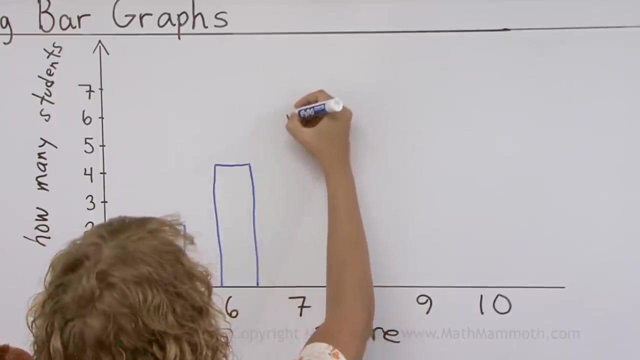 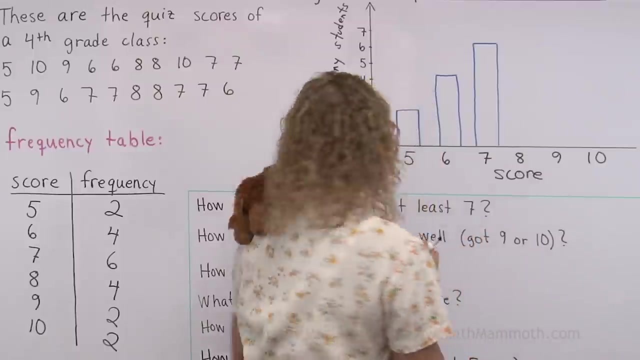 draw the rectangle here, Then how many students got? six Again looking over there, And then four students. So now this time we need to draw it four high, And then seven. Six students- Okay, that's quite many. And then eight points: How many students got that We're here at? 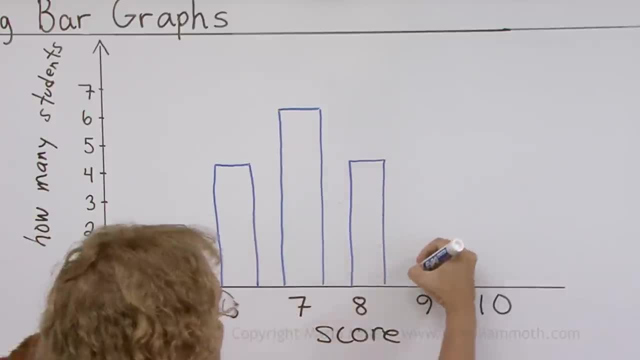 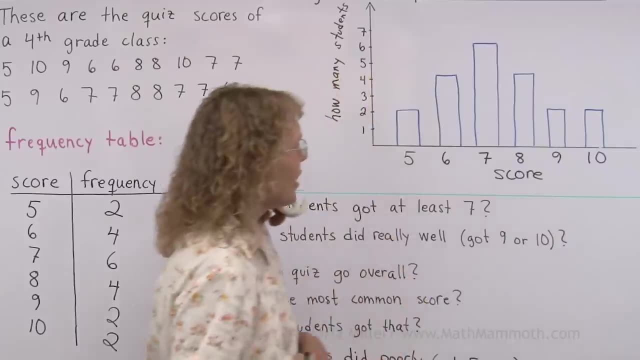 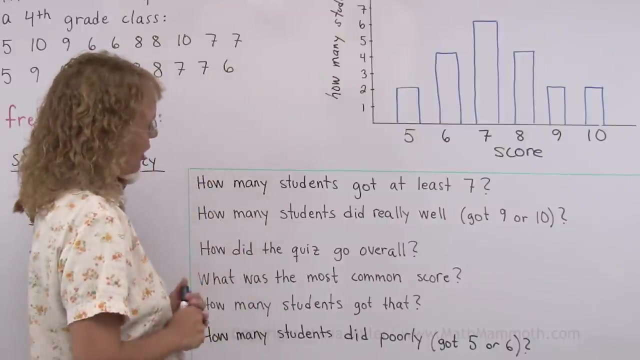 four again. And then, lastly, two students got nine And two students got ten. Okay, And if you want to, you can color these in with pretty colors. Now, lastly, we're going to solve these questions here. They relate to the graph: How many students got, at least? 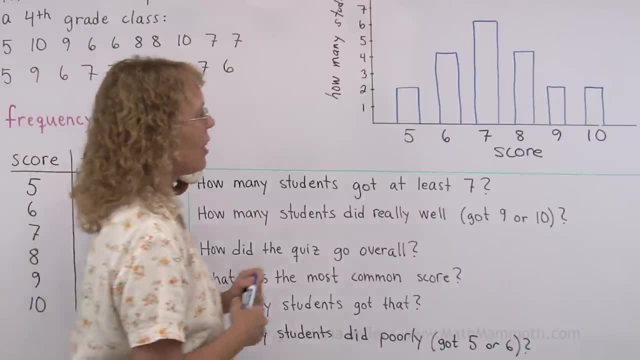 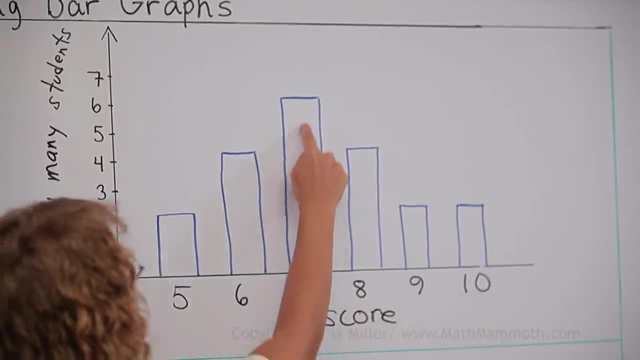 seven, At least seven points. Okay, They got seven points or more. That's what it means: Seven, eight, nine or ten points. So here we have six students and four students and two and two, And you add those. 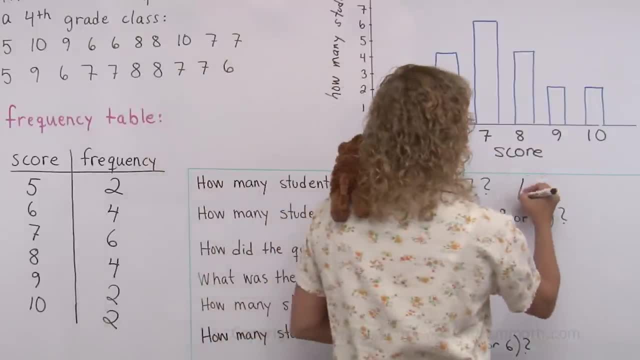 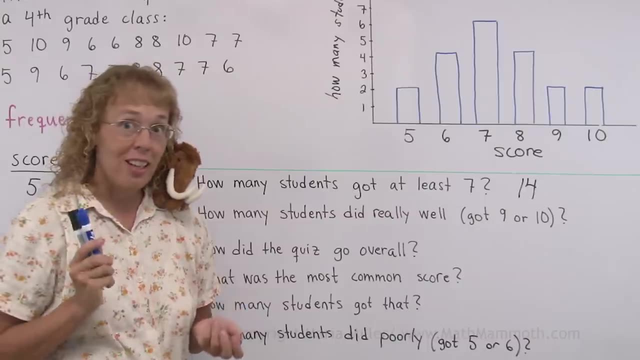 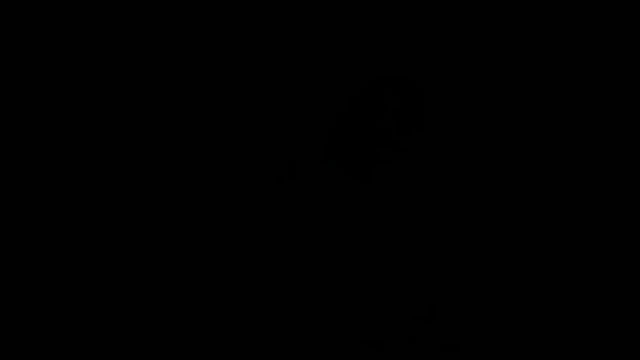 So we get ten, four, Fourteen students got at least seven on the quiz. How many students did really well? They got nine or ten. Okay, These and these, That would be four students, Right, How did the quiz go overall? What would the teacher think, for example, Okay, This. 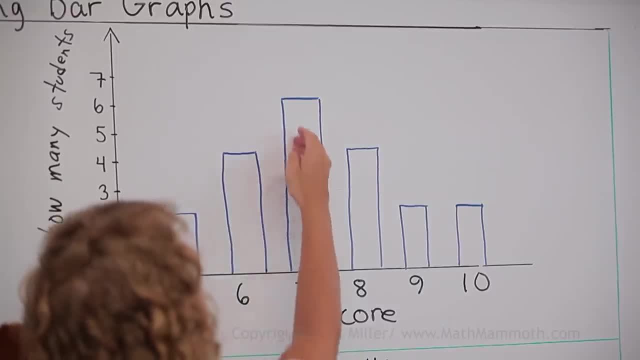 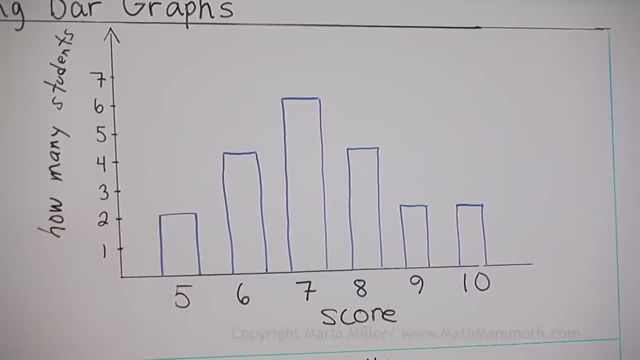 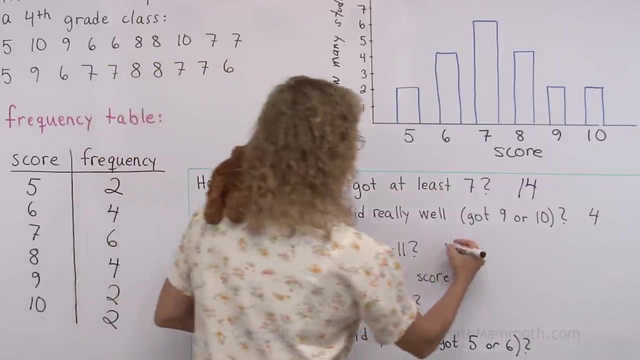 is how the quiz went. We can see that many students got kind of um middle score seven and some got a very good score and some got not so good score. I would say the quiz went kind of regular, normal, usual. Okay, Let me write the answer.